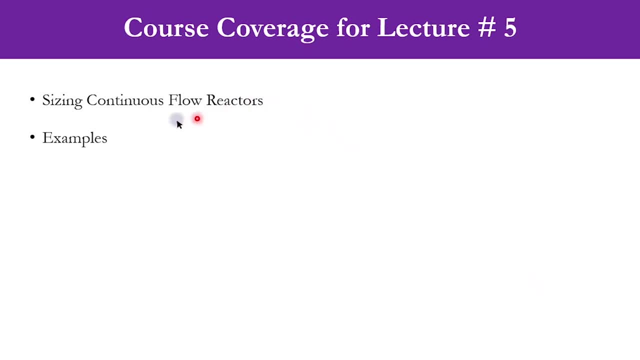 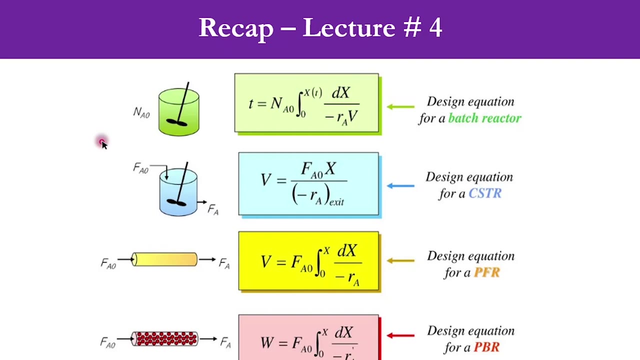 of continuous flow reactors And then we will discuss or we will solve some examples related to sizing the continuous flow reactors. But before going to the sizing we will just have a recap of our lecture number four, that we have derived the design equations for various 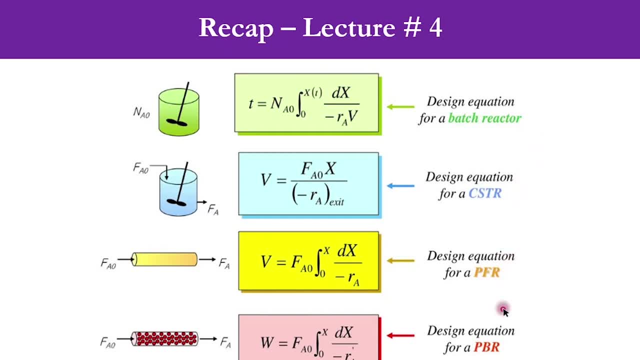 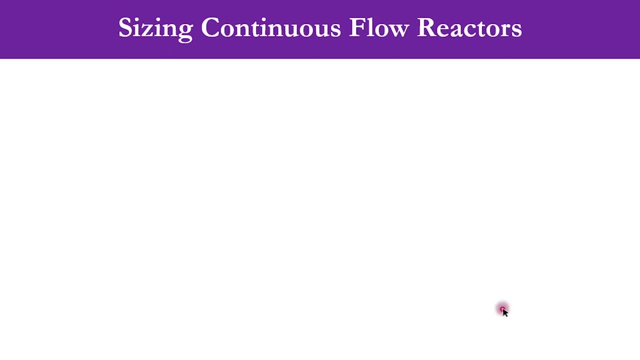 type of reactors, which include batch reactors, CSTR, PFR and PBR. Now, in sizing the continuous flow reactor, the first thing which we will have to remember that the rate of disappearance, or the rate of reaction, is a function of conversion. We will discuss, or we will see it shortly, how it is. 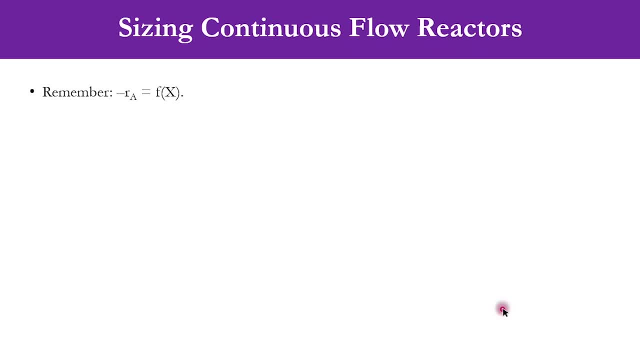 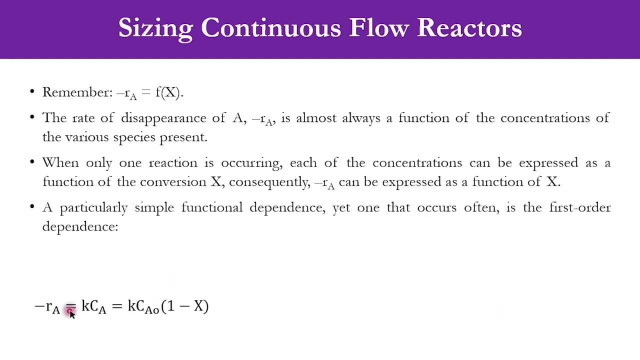 related because we have seen minus RA is equal to KCA, but that's not the case. So we will just concentrate on the function of conversion. The rate of disappearance is almost always a function of concentration of various species present in the system, Like if you see here that for a first, 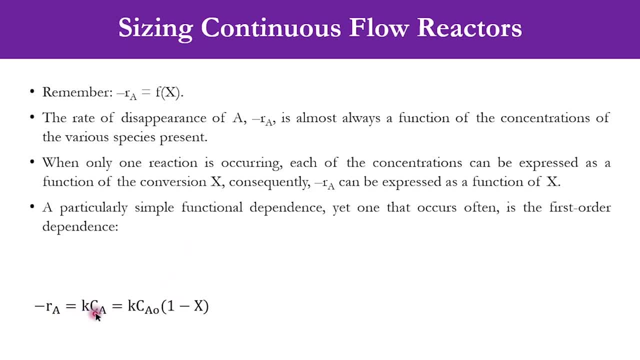 order system it is written as minus RA is equal to KCA And that CA is actually written as CA0 into 1 minus X. So accordingly, once it is written as CA is equal to CA0 into 1 minus X, 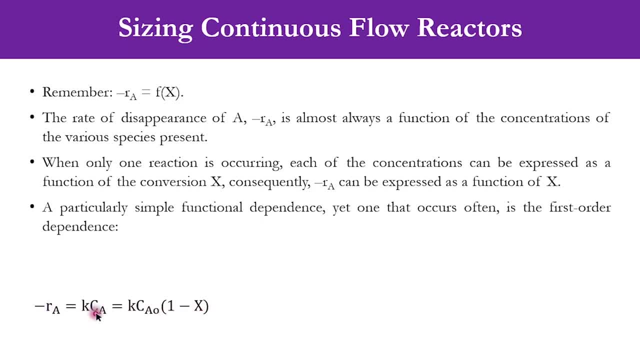 minus RA is a function of X. Now you will be seeing how that equation has been transformed, If you remember that NA is equal to NA0 minus NA0X, which we have used during the derivations. Now, if you take NA0 common from it, 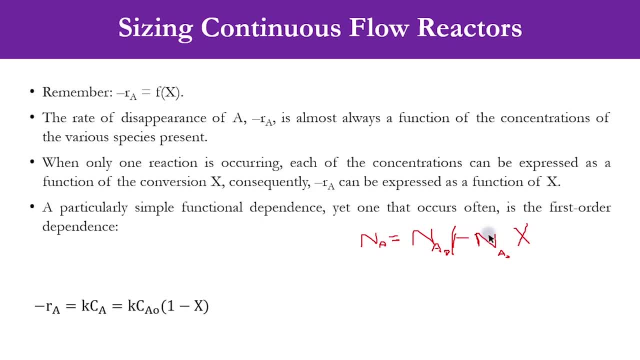 it will become NA0 into 1 minus. this one will be cancelled out: 1 minus X. Now divide that by the volume and you will get: CA is equal to CA0 into 1 minus X. So that is how you derive that expression. 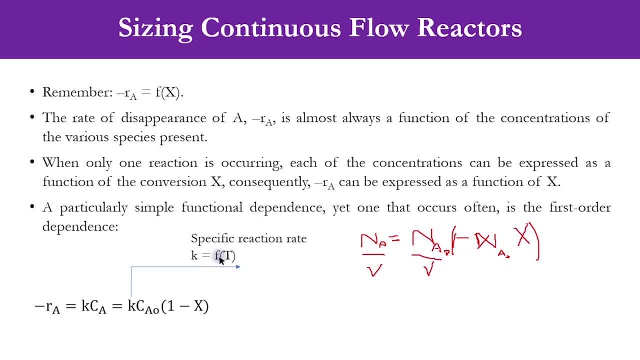 where K is a function of conversion. So that is how you derive that expression. where K is a function of temperature, It is a specific reaction rate, constant. So that thing is definitely written in the slides, but I have just explained it in the lecture as well. When only one reaction is, 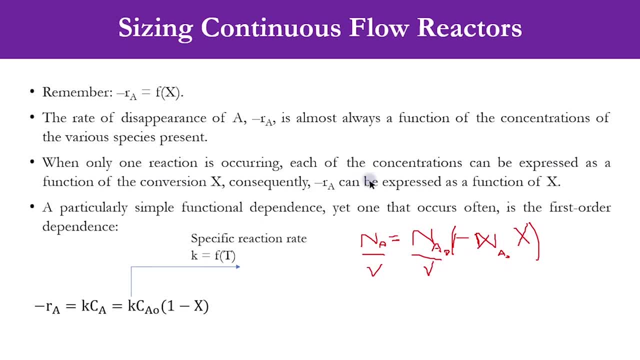 occurring. each of the concentration can be expressed as a function of conversion and it can be written as a function of X. Obviously, for multiple reactions the kinetics will be different. It will be reversible or irreversible in nature. How it will be proceeded once we move to the chapter number 3 and chapter number 4,. 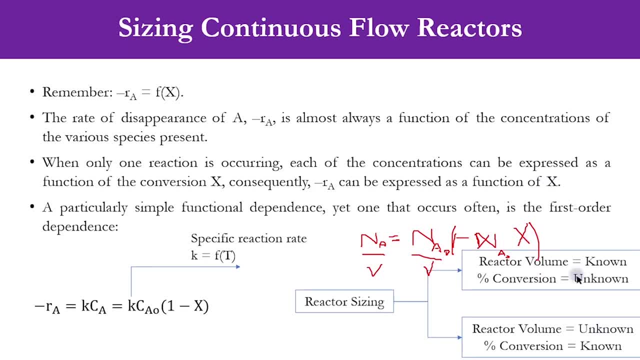 we will see over there as well. During reactor sizing there are two cases or two possibilities. Number 1, we know the reactor volume, but we do not know the percentage conversion. And the second case is: we know the percentage conversion, but we do not know the reactor volume. So obviously one of the 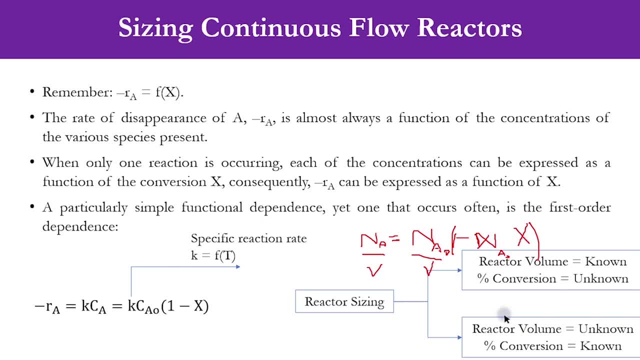 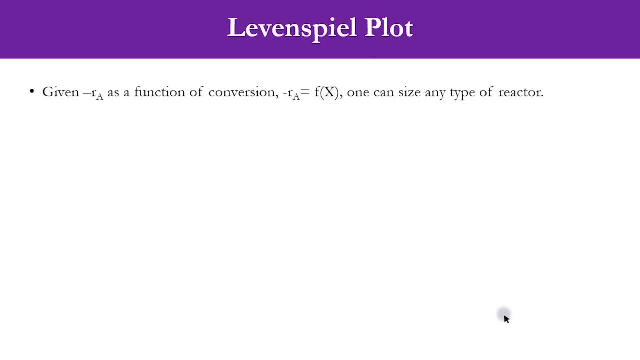 value or the factor is unknown and we have to estimate or calculate it. But before doing that, or before sizing the reactor, we have to get the understanding of the Levenspiel plot, And the starting point is that minus RA is a function of conversion. 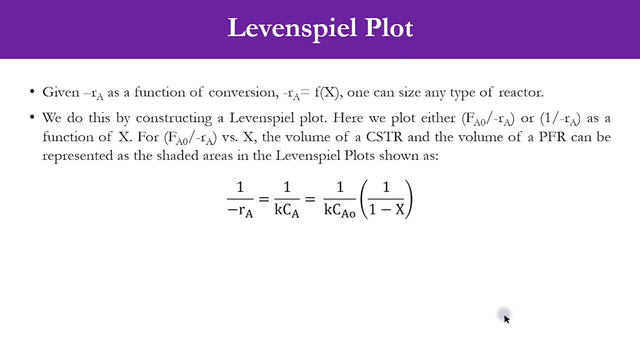 So 1 can size any type of reactor. What we need to do? we need to take the reciprocal of that equation, which is minus RA is equal to k CA. That will become 1 over minus RA and that is equal to 1 over k CA and CA will be equal to CA0 into 1 minus X, So that will become as 1 over k CA0,. 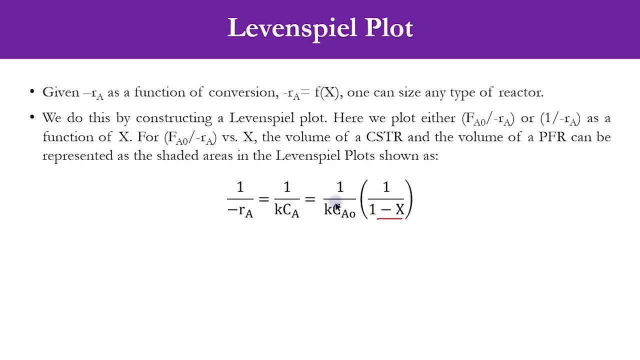 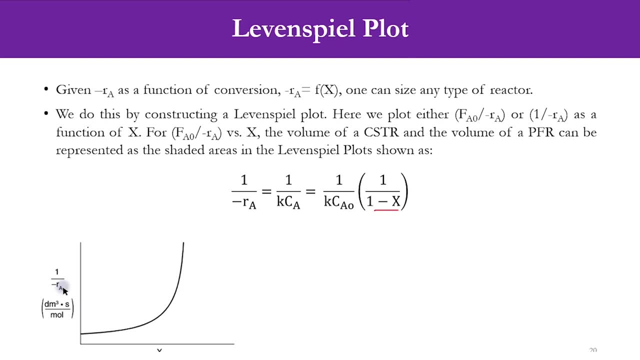 1 over 1 minus X. But now, after doing that plot, there are two basically plots that are included. Number 1 is the plot of conversion versus 1 over minus RA And accordingly, you see, the plot is generated over here. And the second plot is between X and FA0. 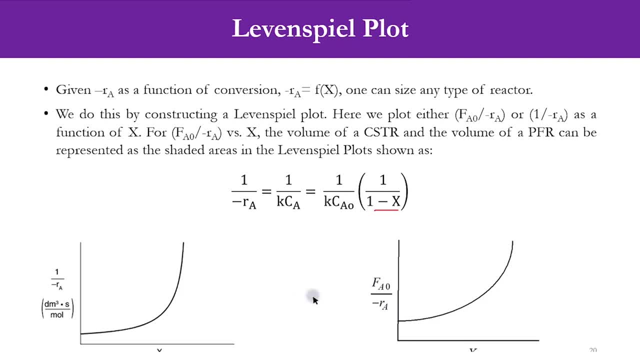 over minus RA. Now you can see that both plots are actually the same in nature. The only difference is this value of FA0, which is not present over here. But you see, the trend in both the cases will remain the same And once we go to the example, we will also solve it over there as well. 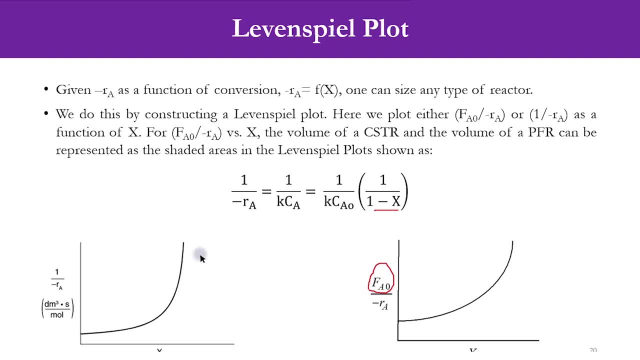 So what we need to do, we need to first draw the Levenspiel plot. once we are graphically the volume of the reactors, the sizing are being done for the continuous flow reactors, that we have to plot either FA0 over minus RA or 1 over minus RA as a function of X, And then we can calculate. 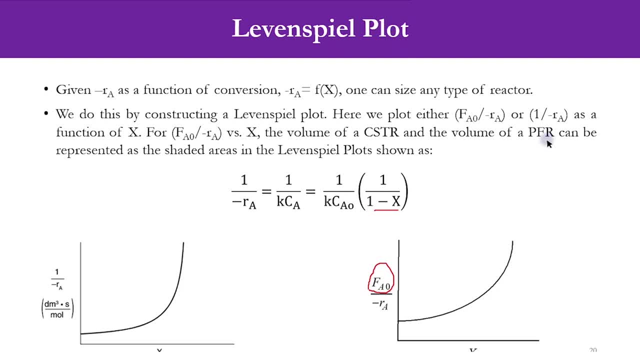 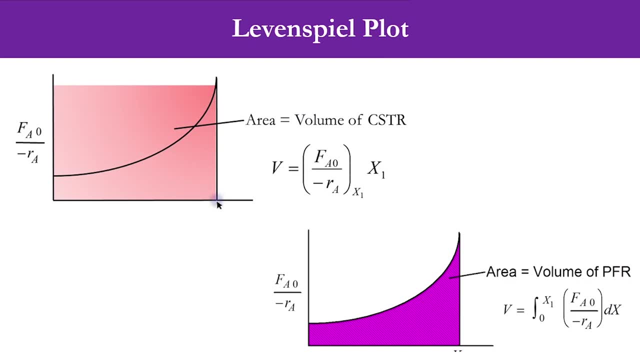 the volume of CSTR and volume of PFR. Now the question arises how we can calculate- So this is the answer in this slide- that what you need to do. you need to take one point, For example. this represents X at somewhat like 0.9.. You have to draw a straight line over here. 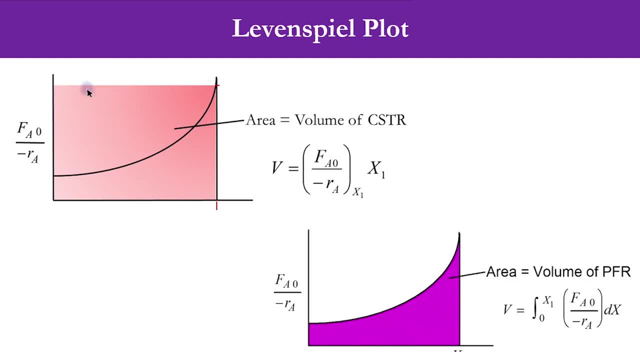 And that will connect with this curve over here, And then plot a straight line which connects this Y axis And the area. this area complete area- will represent the volume of CSTR, While in case of PFR it will be the area under curve. So that is the main difference between volume of CSTR and volume. 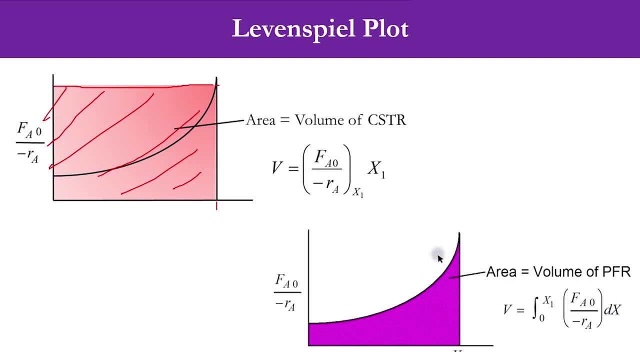 of PFR. Now, if you summarize it, basic summary is that you have to first draw. the Levenspiel plot could either be FA0 over minus RA as a function of X or 1 over minus RA as a function of X And based. 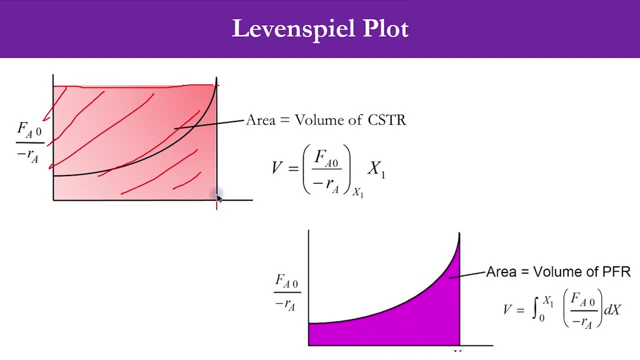 on plot which has been obtained. if you want to calculate the volume of CSTR, what do you need to do? For example, if you want to calculate here, then simply draw a line here which touch it, and then draw a line here, And this area will be the volume of CSTR. On the opposite side, the area, 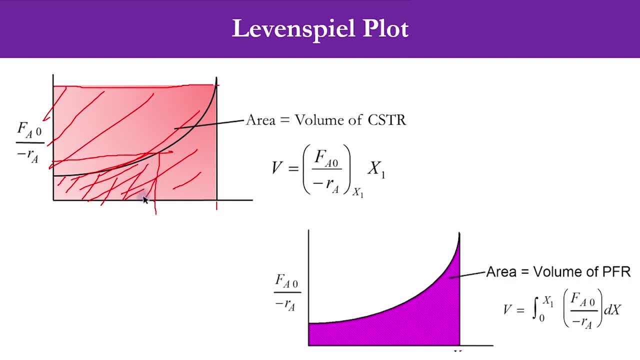 over PFR. So in that area- or let me, I am going to do it to PFR, In some cases I will do it to PAFR failing because they are now other categories, other categories in the unit, So they are not obtained and they sometime they are done from broader. 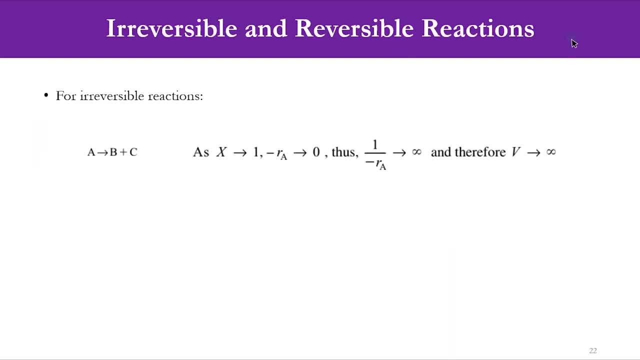 organization. So this is for. Doesn't it make sense, Can youzić? I like this. We will arise this new case here. So we have this here. You can see that the volume of PFR varies in raineds게. 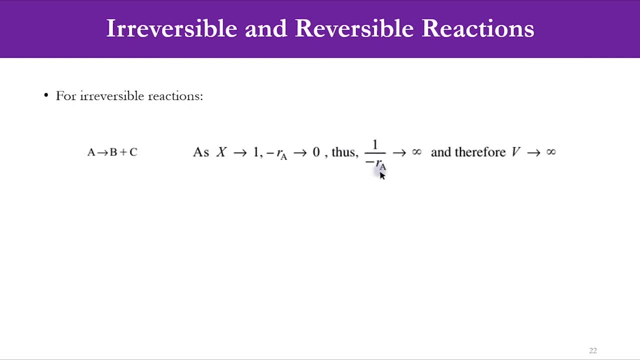 one, the rate of reaction minus rA approaches to zero. accordingly, one over minus rA approaches to infinity and volume will be infinite. which will be required for this, while for the reversible reactions, which we say A goes to B plus C and B plus C can react to form A, the maximum possible. 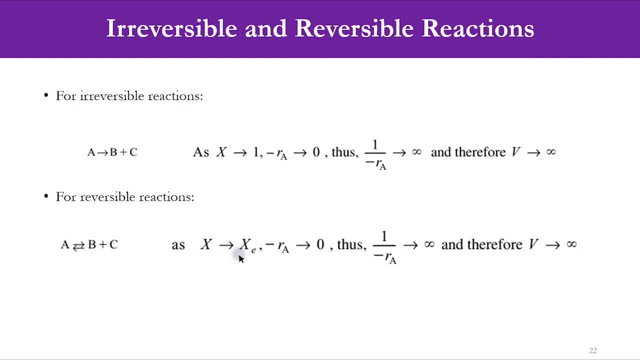 conversion is equilibrium conversion, as we have discussed in our previous lecture as well. minus rA will approach to zero. accordingly, one over minus rA will approach to infinity and volume will approach to infinity. so infinite volume is required at equilibrium conversion for the reversible reactions, and for the irreversible reactions infinite volume is required to make. 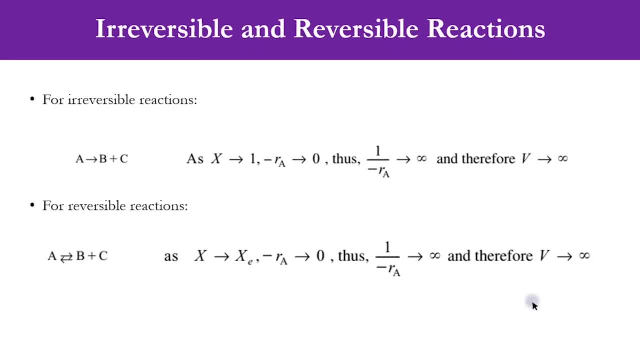 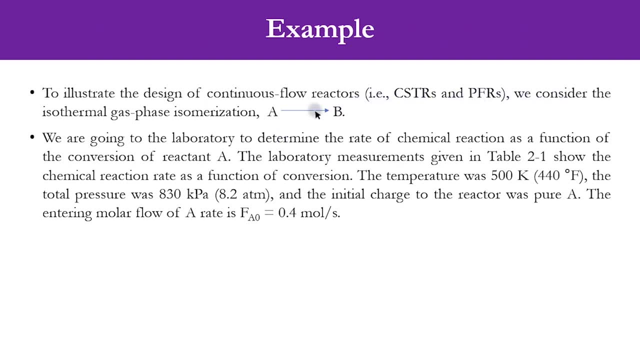 100% conversion in the system. now, moving on to the example which we will be doing today, that to illustrate the design of continuous flow reactors such as CSTRs and PFR, we consider the isothermal gas phase isomerization, in which A goes to B. we are going to the laboratory to determine. 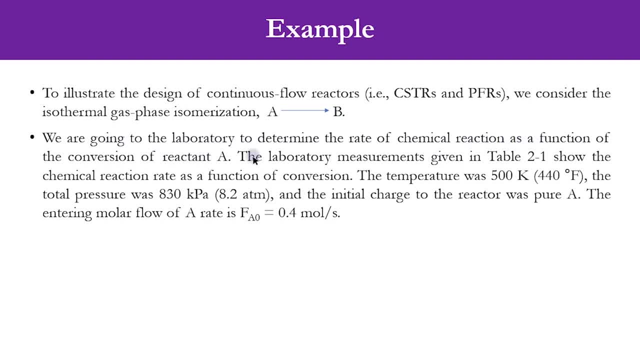 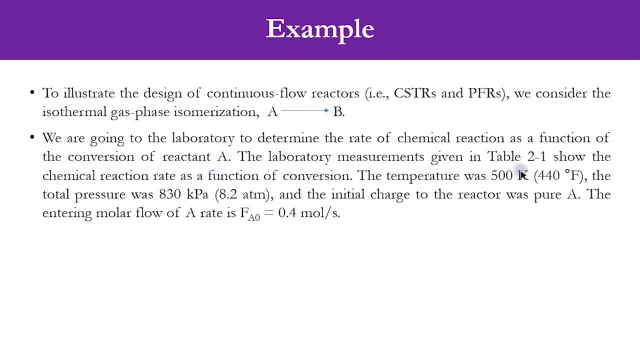 chemical reaction rate as a function of conversion. the temperature was 500 kelvin for 40 degree fahrenheit, the pressure was 830 kilopascal and the initial charge to the reactor was pure A. the entering molar flow rate of A is: FA0 is equal to 0.4 mole per second. so you can see that you. 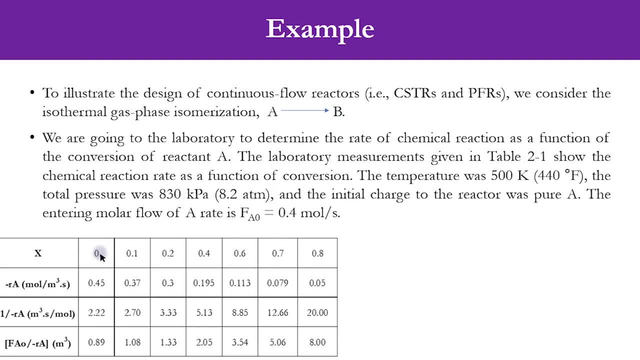 have been given the values of x at 0.1, 0.2, 0.4, 0.6, 0.7, 0.8, and correspondingly, values of minus ra are not given. so what we will do? we will go to the excel. 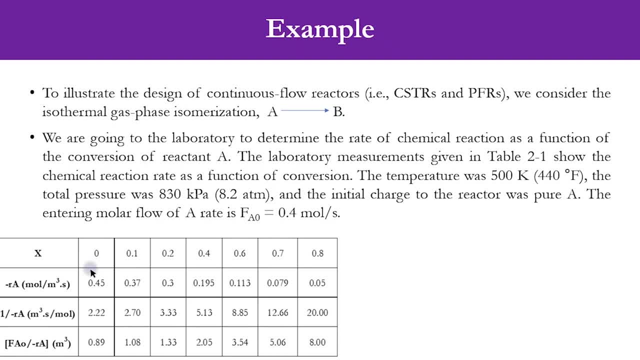 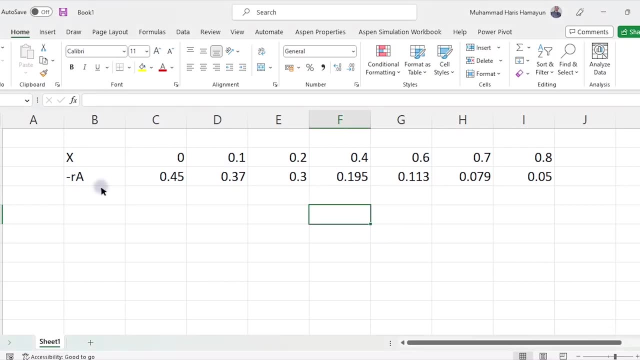 now, and we will draw the levinspiel plot under two conditions: one is for 1 over minus ra and second one is for fa0 over minus ra, and we will see whether these two plots are same or not. so now we are moving to the excel sheet and the data for x and minus ra is given to us now. first we need 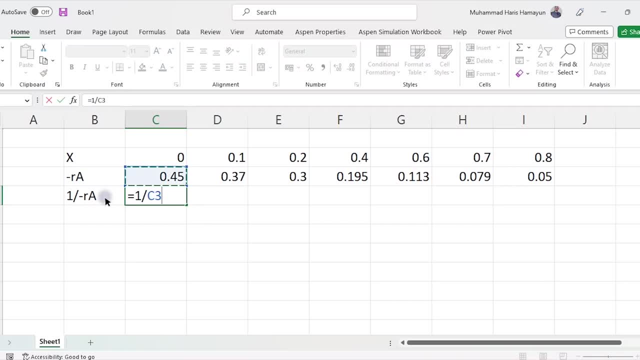 to calculate one over minus ra, and that is simply one divided by this value. so, and accordingly, we doing the copy paste over here and the formula will be copied and you can see we have got the plot. simply using number system to get it to two decimal or maximum, we can get it to three decimal. 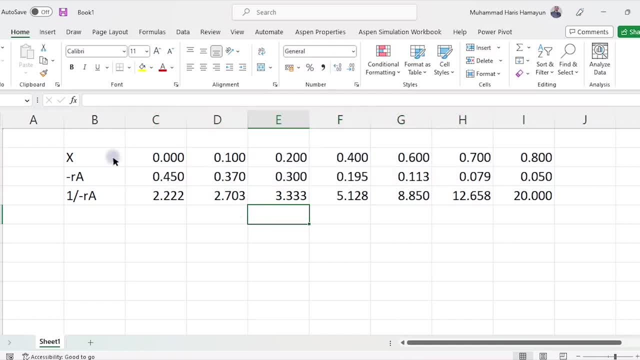 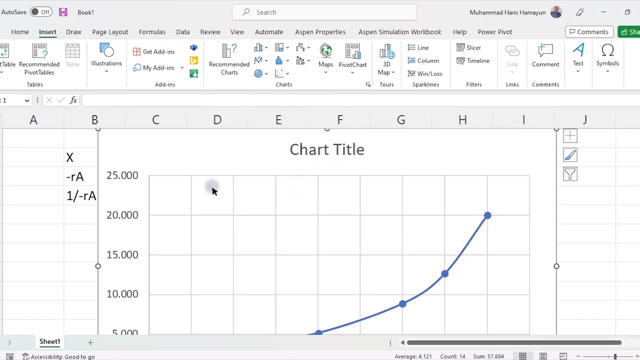 using this vector. Now we have to draw the plot between x, which is at x-axis, and 1 over minus r, which is at y-axis. So what we need to do, click it, press control from keyboard, select it, go to this, insert charts and the plot is generated over here, which represents the 11th scale plot, and 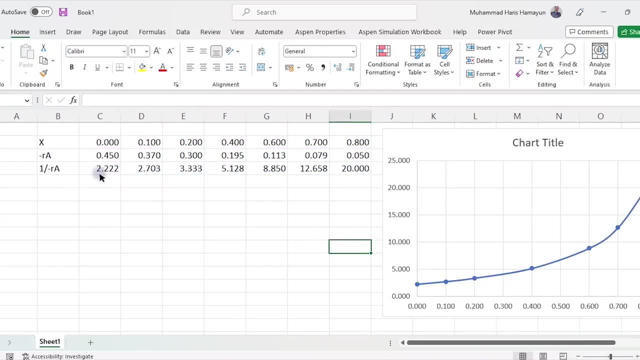 accordingly, you can see x versus 1 over minus r a. plot is generated for the system. Now we know that fa0 value is 0.4 mole per second. so what we need to do? fa0 over minus r a and simply multiplying 0.4 with this calculated value. So accordingly, just drag it over here again, giving it just. 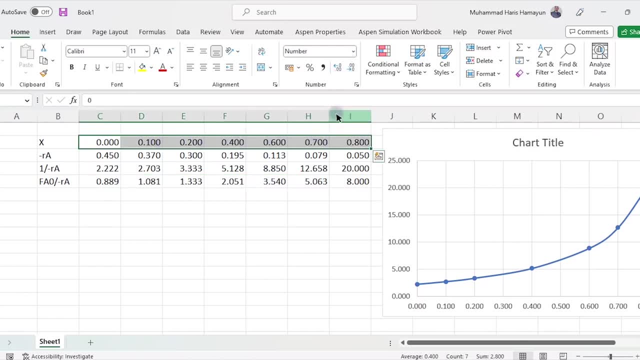 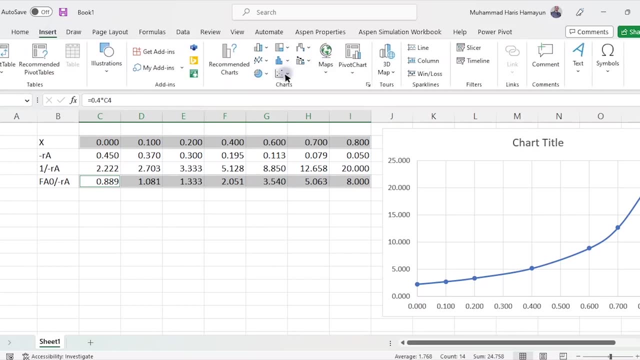 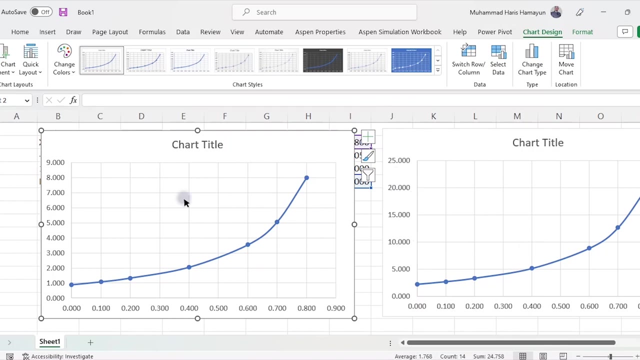 three decimals. and now in the same fashion. it is simple mathematics, so I'm doing it very quickly: press control from the keyboard again, select it, go to insert charts and you can see. now you can simply see that both the trends are same. only there is a difference in the y-axis values. but the trends will remain the 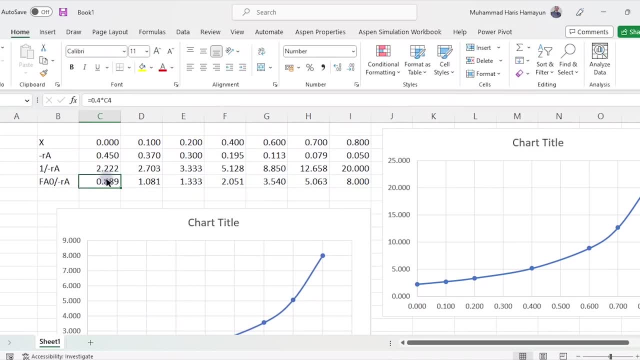 same because mathematically, if you see only 0.4 as a factor, is multiplying over here. so the trend which will be generated with 1 over minus r a will be the trend which will be generated for the system. So the trend will be 0.4 over minus r a. so, using either this or this will surface for the 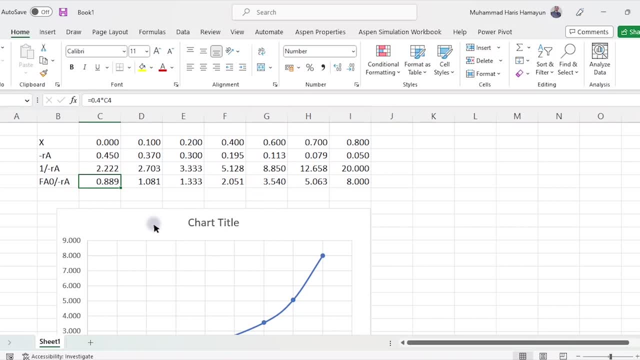 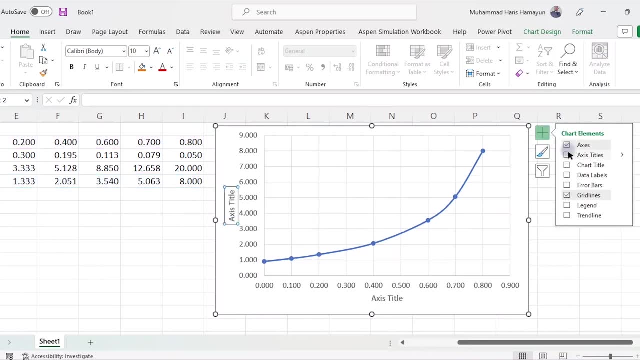 calculation of volume of CSTR and PFR. So let's see, we select this one which is fa0 over minus r a, and obviously the other parameters can be like. we can give axis titles, and this one is x and this one is fa0 over minus r a, and the unit will be cubic meter. So once we have generated it, now we have to find 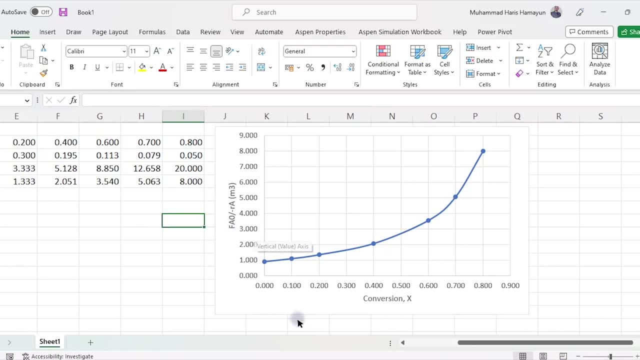 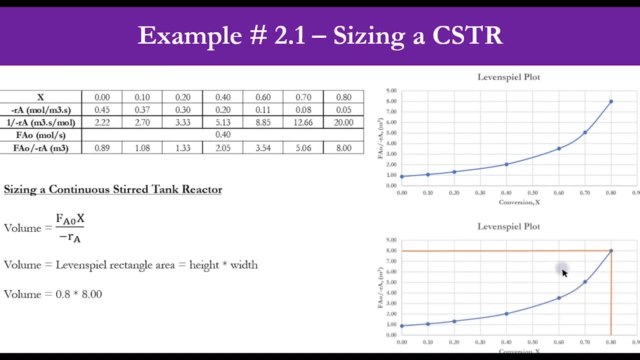 the value of volume of reactor, as in the next statement. if you see here that for the Levenspiel plot which we have been generated in the previous example, we have to size the CSTR now. and for the CSTR what we need to do, we need to take point from here, connect it to the line here and then plot line. 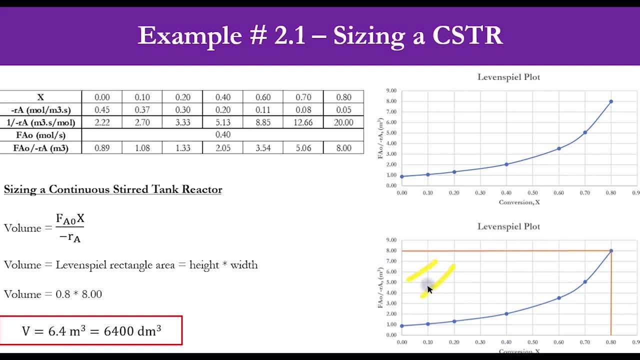 here and this area. if you see here and this area, the rectangular area will represent the volume of CSTR in the system. So by multiplying 0.8 here with the value of 8, multiplying these two values will give the answer of volume of CSTR at a conversion of 80 percent. Similarly, if we want the value at 40 percent, simply, 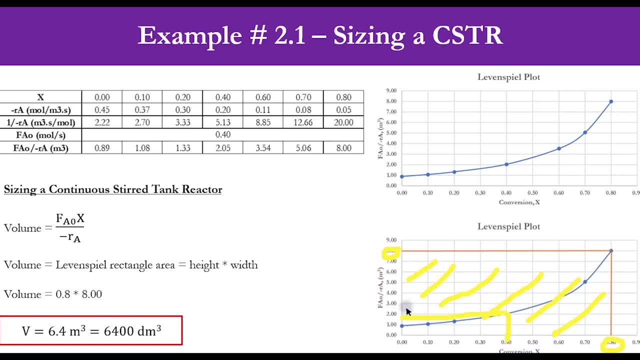 take a line from here. take another line from here at somewhat about point at 2. so accordingly, do multiply by 0.4, so approximately 0.8 cubic meter or 800 cubic decimeter value will be required for the system. So now what we need to do? we need to go back to Excel and we need to go back to the 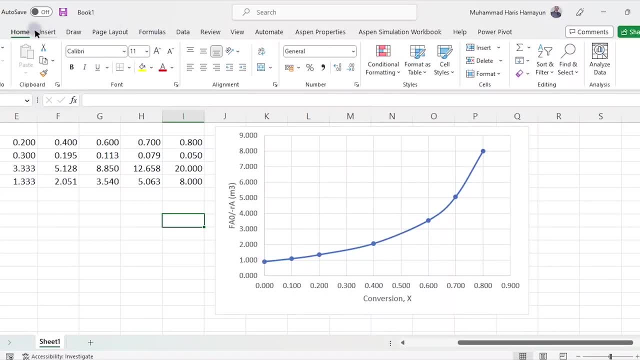 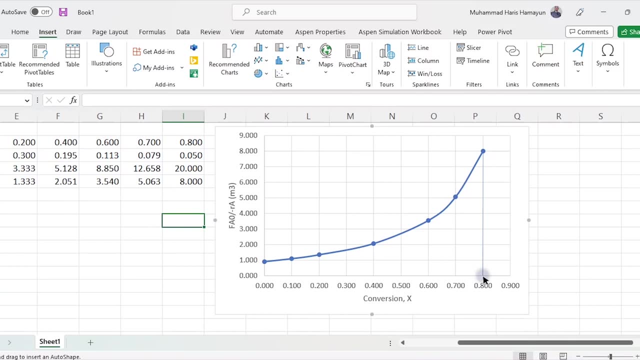 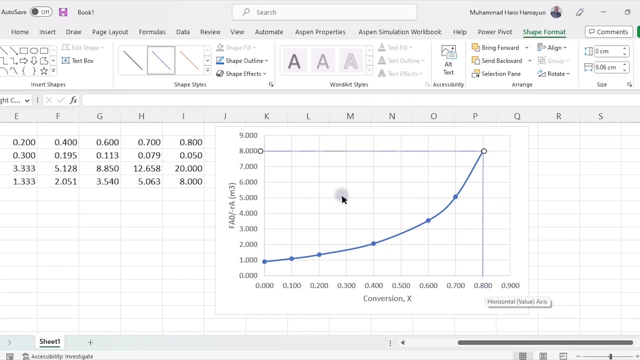 and now you see you have got this plot. simply what you need to do here, that you need to go to this illustration in shapes and let's see that you draw a line over here and then simply take a line straight line over here and this area, which represents the volume of CSTR Now multiplying-